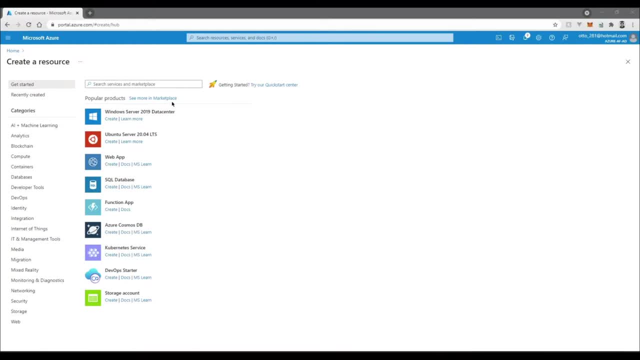 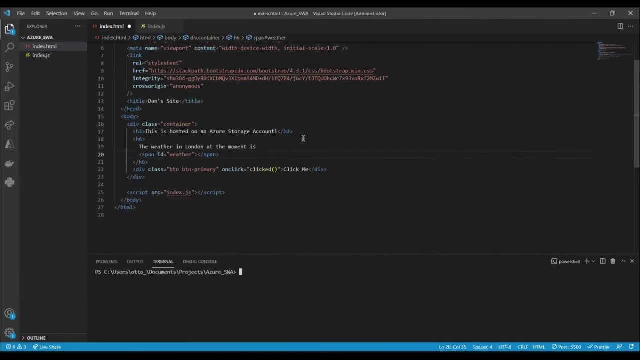 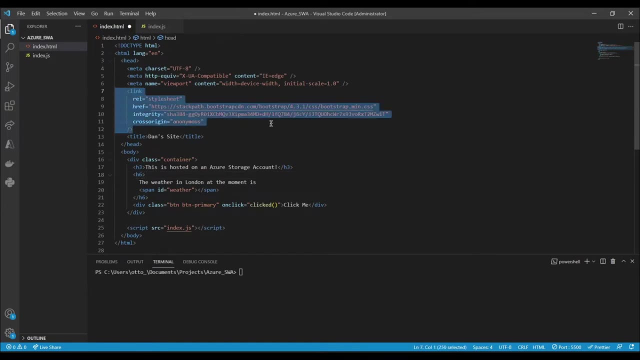 Hey, what's up guys? today I'm gonna be running you through how to set up a static website using Azure storage accounts. Now, I've already got a basic HTML file right here. All it has is just, you know, a title, a couple headings, and I've imported the bootstrap CDM for its CSS. so it's style sheets for the. 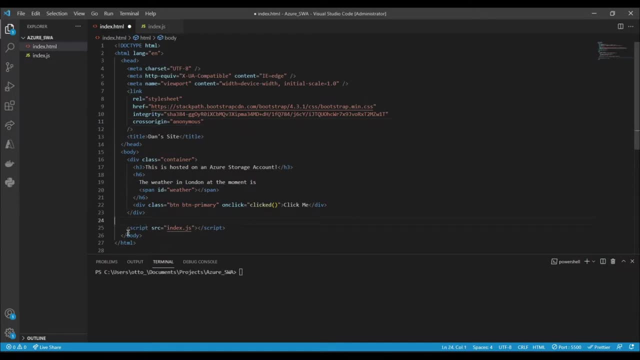 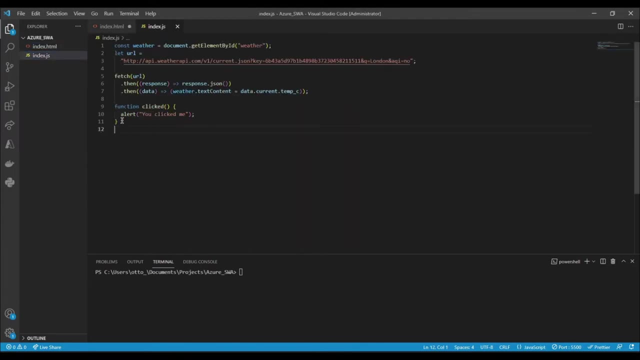 bootstrap. On top of that I've also got a small indexjs file which I've created, and this is just to highlight some of the limitations of the storage account, and you'll see in a second. But basically all I'm doing here is just making a call to a public API which returns back some weather data. 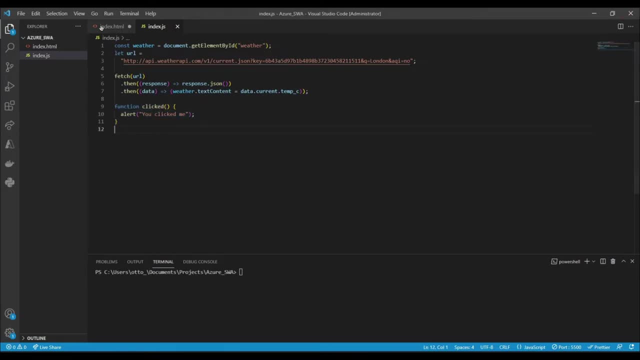 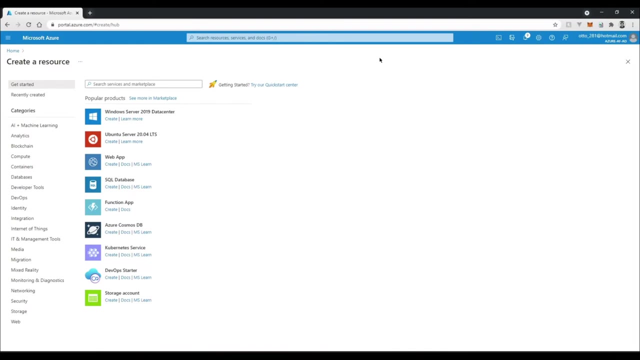 and then I've also got an alert function here for a button click. So you'll see all that in a second. but first off, let's actually go back to our Azure dashboard and create a storage account for the hosting. So just from here you can go storage account, I think, and we. 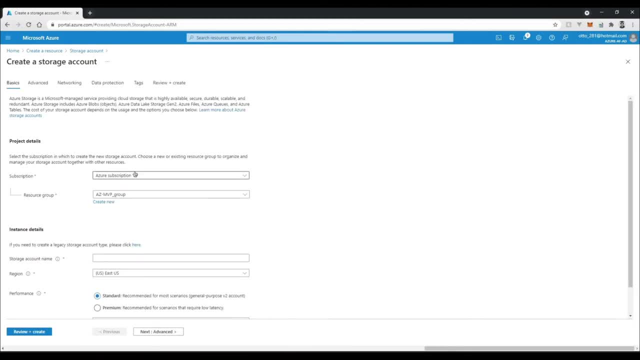 can just go create. Now we pretty much can leave all the defaults the same. just make sure you've got an active subscription and just pick whatever resource group you want to assign this to. or you can create a new one just to encapsulate the video in this tutorial. You can call your storage account whatever. 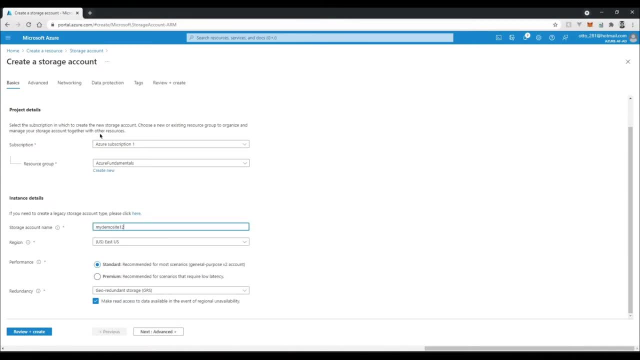 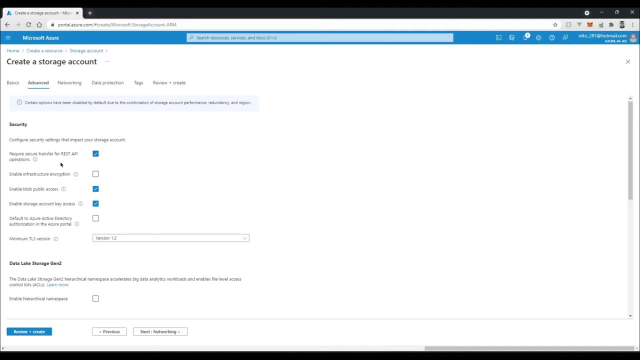 you want. so I'll just say my demo site one, two, three and pick the region closest to you And the rest we can basically leave the same. we don't need to worry about any of this stuff here. access to your as hot, that's fine, and making sure that the endpoints are public for all. 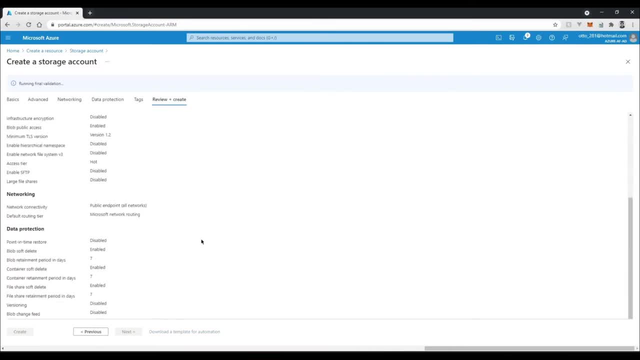 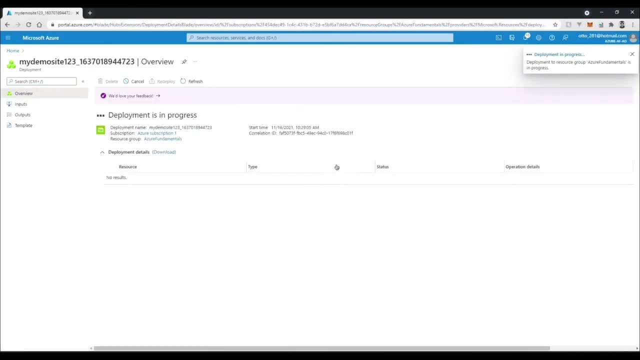 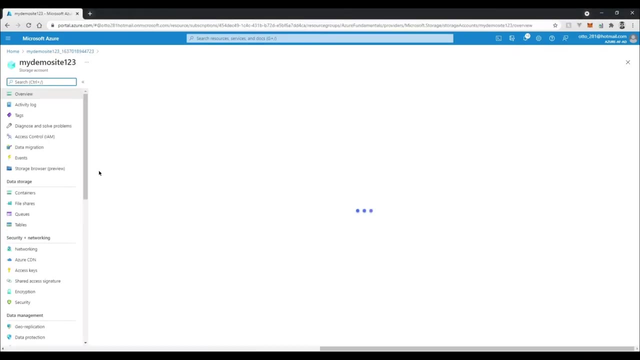 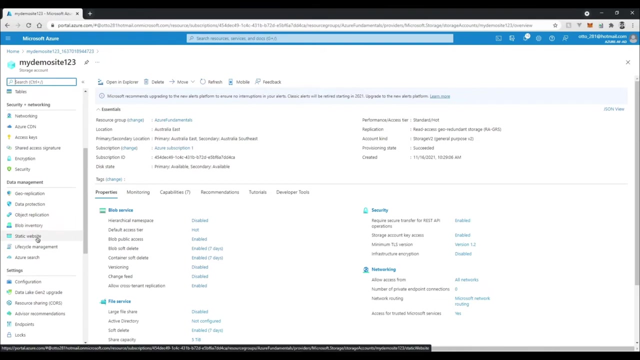 networks for today's purpose, Anyways. so just review and create. validate first. once that comes back, create it. Alright, now that's going to take a second to deploy Sweet. so once the deployment is complete, go to your resource and just scroll down, and all we need to do is go to the static website section right here. 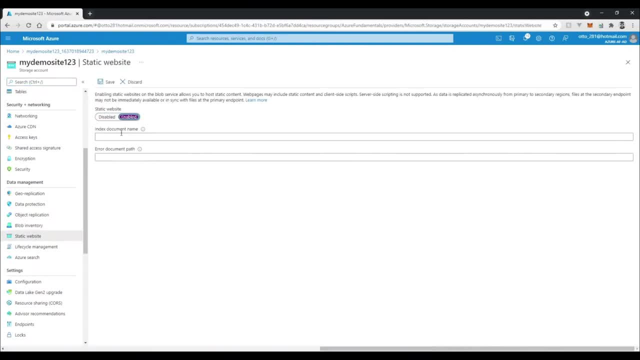 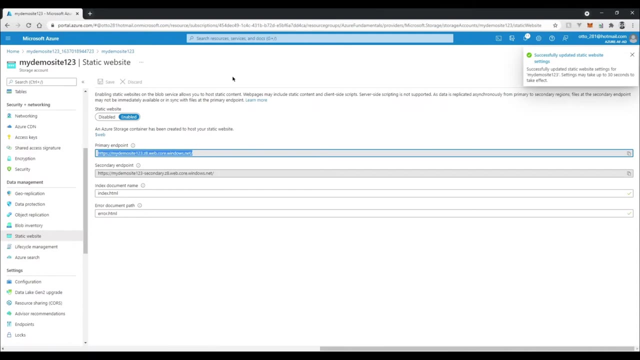 so click on that And we'll enable this and the index document name. so this is the entry point for the website and then the error document as well, in case there's an error. I'll just say this away, and this is our end point: to actually access the website. 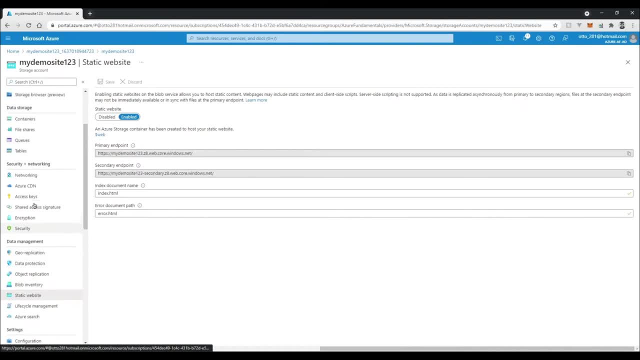 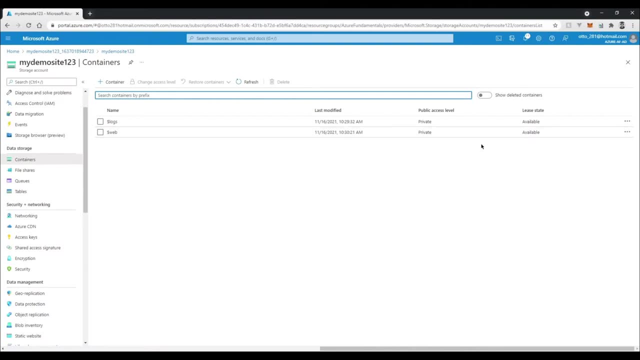 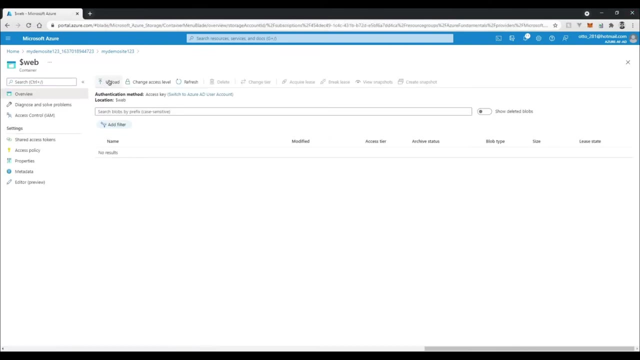 So before we actually go there, though, let's just go up to containers, and you'll see, here it's now generated some two containers for us, so one for the web files and then one for the logs, And we want to just add some stuff to the web container, So we'll just upload here and I'm just going to select. 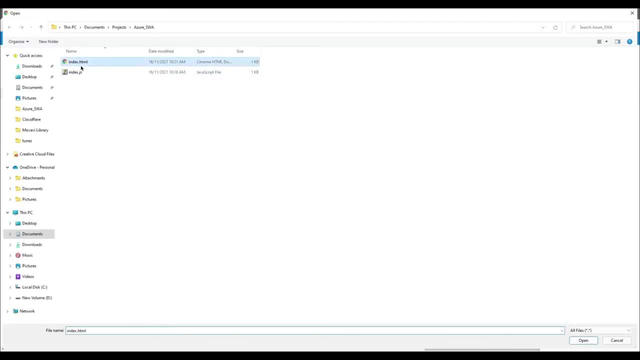 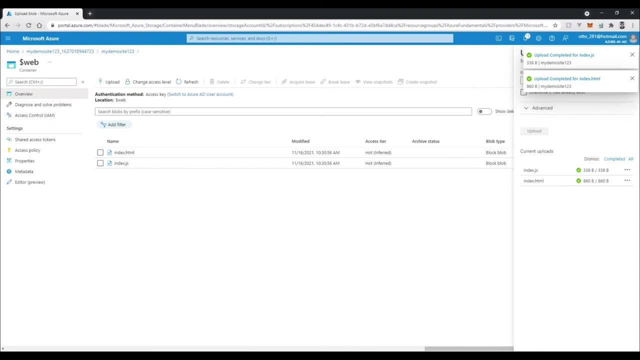 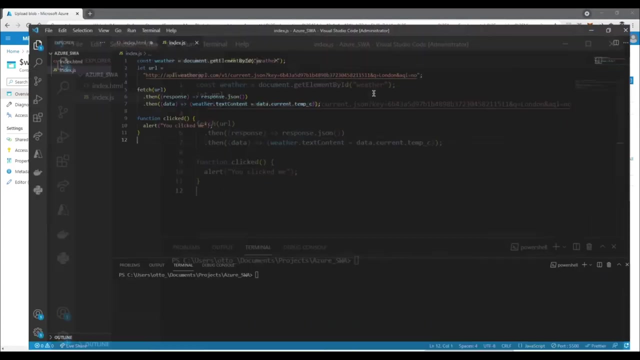 those two files that I already have, So the indexhtml and the indexjs. I'll put them both in and I'll upload that. So before I actually go to the website now hosted by Azure Storage, I just want to show you something first. So this is the website here running locally for me. So I've got. 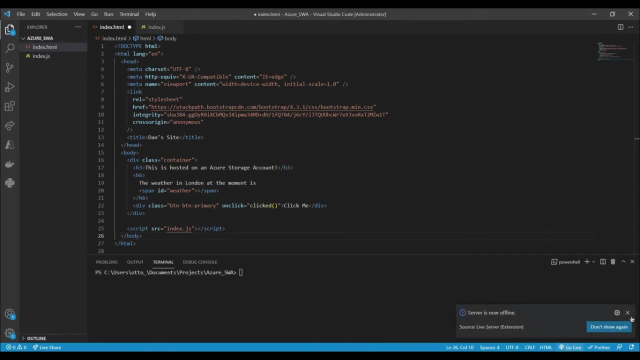 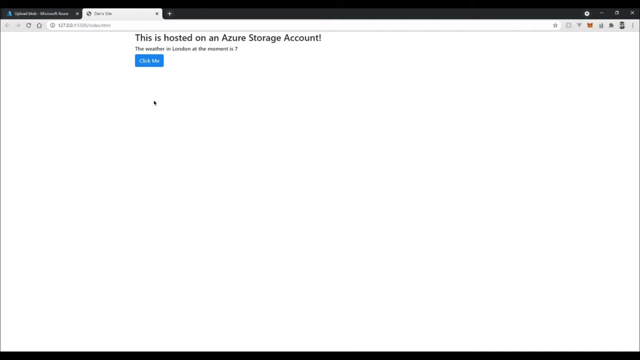 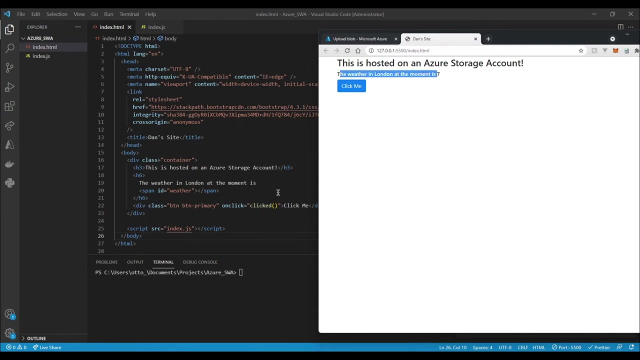 it running on local server at the moment, so I'll just close this off and I'll start it back up again. So this is what the website currently looks like. right, It's just a basic header. This is hosted on Azure Storage. The weather in London at the moment is, and then degrees is. 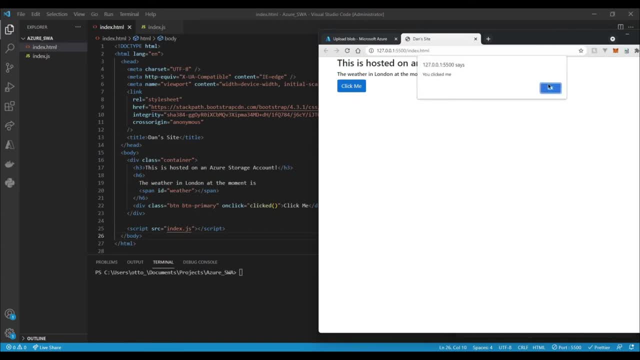 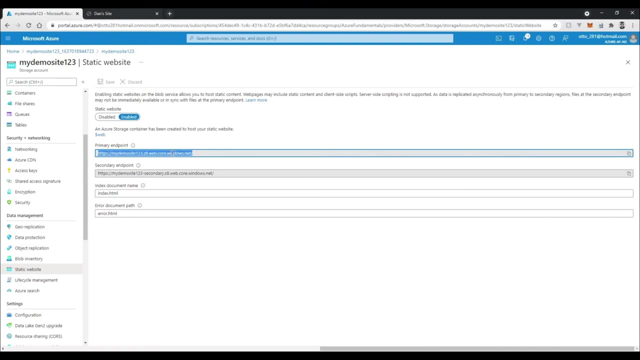 captured from the API and then there's click me alert Now. so this is all working fine on my PC, It's working locally on this live server. but now if we actually go to the storage, So if I go back to my endpoint that I have, I just copy this over. If I just copy. 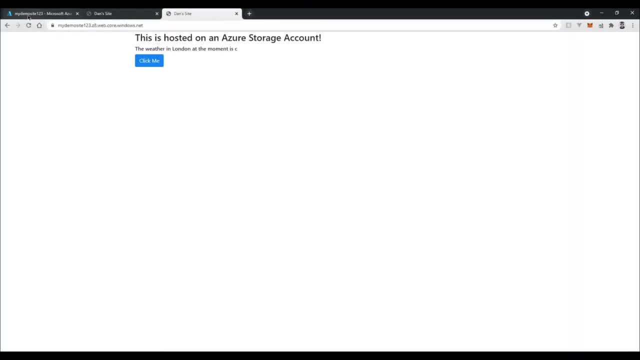 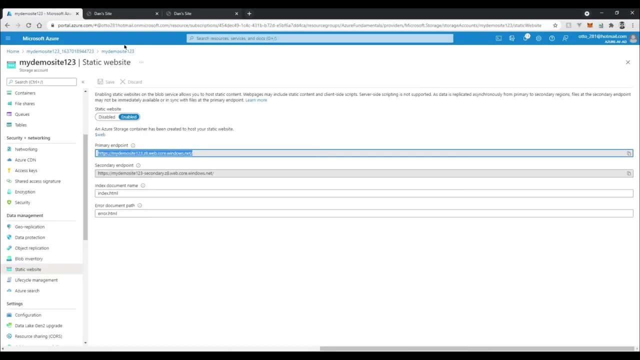 this and then paste it in. you can see now that the API data isn't being called, and that's because Azure Storage cannot handle dynamic data, So it can only handle static content, right? So all the stuff that we've loaded there is fine for it to use. it can handle that, but as soon as we try to request data from a external source. it can't handle it, So I'll just go back to my window and I'll go to the storage. So now, if I go back to my endpoint that I have, I'll just copy this over. if I just copy. 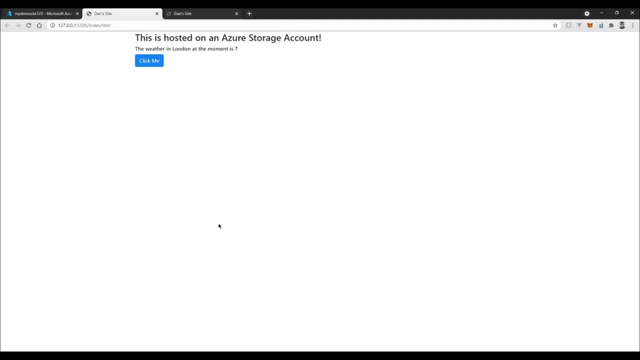 this and then paste it in. You can see now that the API data isn't being called and that's because Azure external web server it's gonna basically fall over, so but this, this function here, will still work on the edge of storage. so if I click this, that still works. 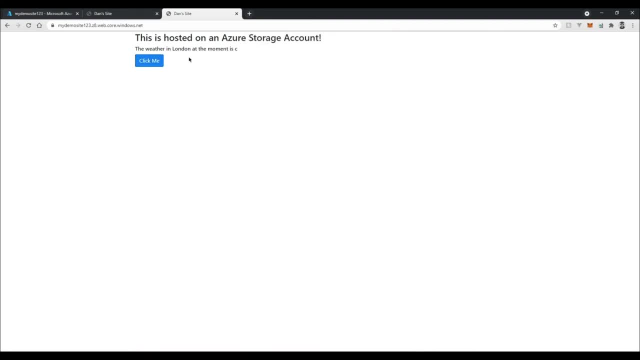 because that's not pulling external information from another web server, whereas um the way the data is. so that is just something I want to highlight. otherwise, guys, that's pretty much it. it's a pretty quick example. I guess the use case for this, if you're wondering, would be if you are hosting static stuff.